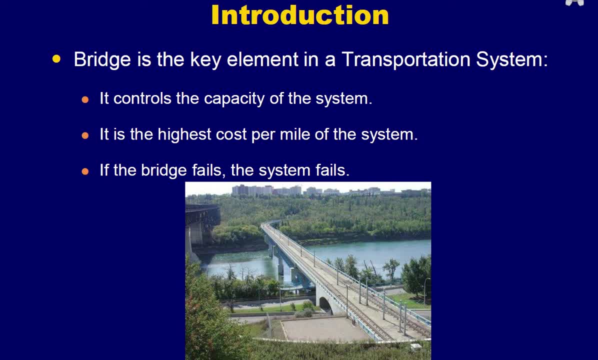 the system. if the bridge fails, the system fails. okay, so, for example, you have a road. let me show you the, explain you the figure. for example, the road is coming from this side and continuing on this side. this is the bridge. now the per unit cost of road over here and per unit cost of road over 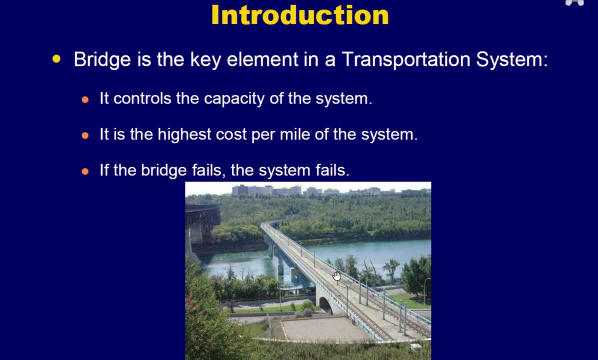 here will be much more lesser than the per unit cost of road or in this span length, because of the construction of the bridge. okay, so it is the highest cost per mile of the system. it controls the capacity of the system. for example, if the road width is four lanes over here and four lanes 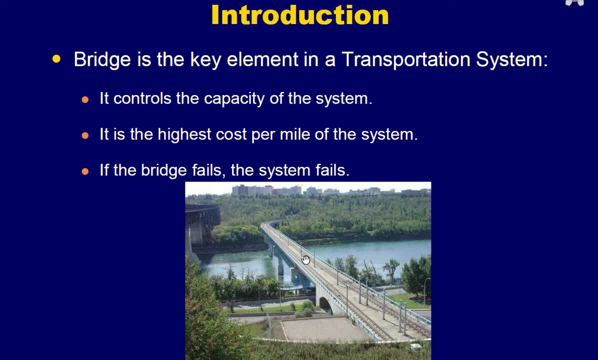 over here and you have constructed a two-lane bridge, so the purpose will be failed, because the the traffic coming from this side, the two lanes will be submerged into one lane and they have to wait over here. similarly the case the traffic coming from this side have to wait over. 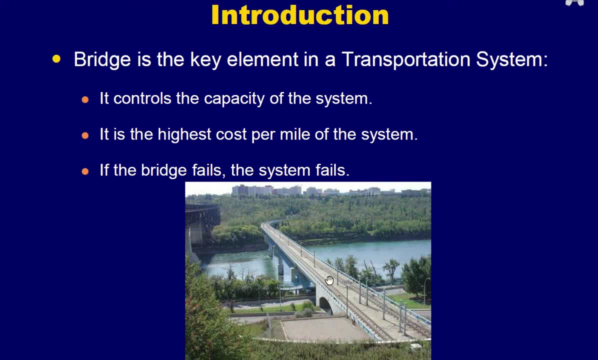 there. so if the bridge is of not the equal span of- sorry- the the equal number of lanes or to that of the adjoining roads, then it is of no use. so the bridge controls the capacity of the system. it is the highest cost per mile and if it fails, the system fails, because if the bridge fails, the road will be. 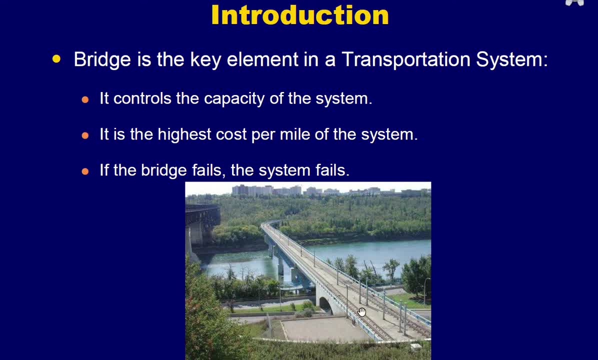 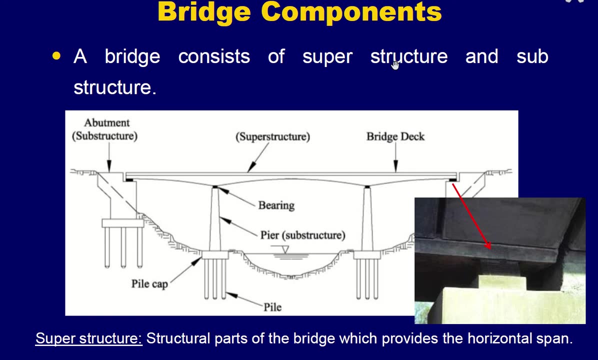 of no use. so the the 20 kilometer or 100 kilometer road will be of no function if this small portion fails. so this is the key element that need to to be designed and analyzed carefully. these are some of the basic components of a bridge. a bridge consists of superstructure and substructure, and what are 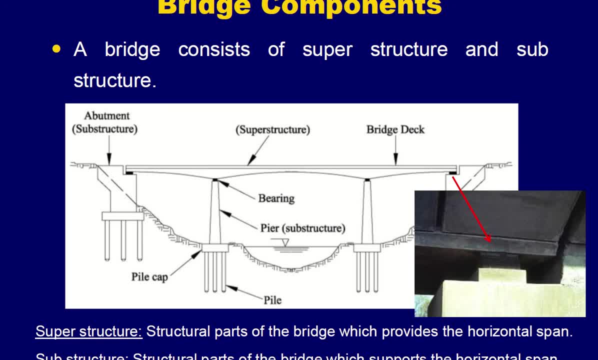 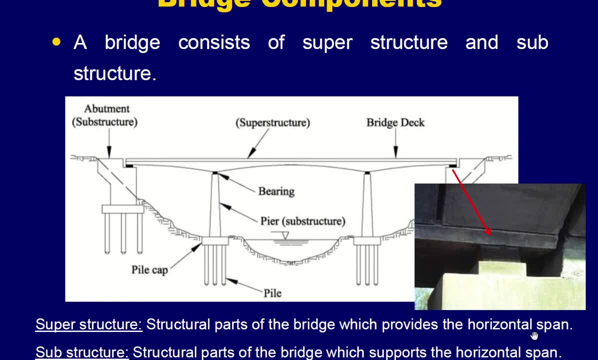 superstructure and substructures. you can see that superstructure are the structural parts of the bridge which provides the horizontal span. okay, substructure are the structural parts of the bridge which supports the horizontal span. so so the Minted structure over here. This is your superstructure, right. 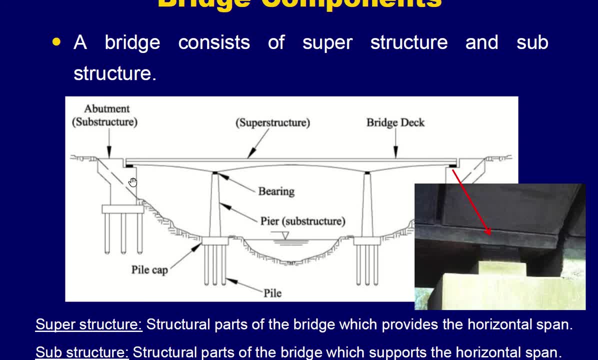 This is, or here, this is your super structure, right and beneath these are the sub structures helped to build a bridge. If you look to the, the upper crown of the bridge, this is the horizontal span. this is called the superstructure, okay, and the the components that are supporting the superstructure: the piles, the Pile forge. 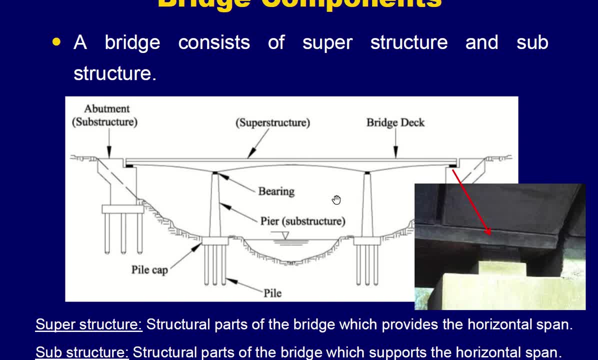 Pior, the buildings, everything. these are substances. Okay, The abatements are sub structure and this deck and girders. If, If there is an energy shortage issue in this process, jogar1 should be finished and when there is a 40 $ kill. this is the main advancement in infrastructure. So this, the main differences between two points are: what is the structure and the terminal control? is котором quality? namely, this is a super structure. okay, Take a look and see if there is a vehicle over here. this is your infrastructure. right and below, these are structures. 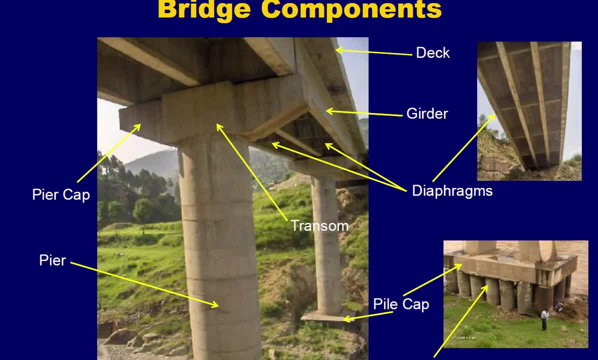 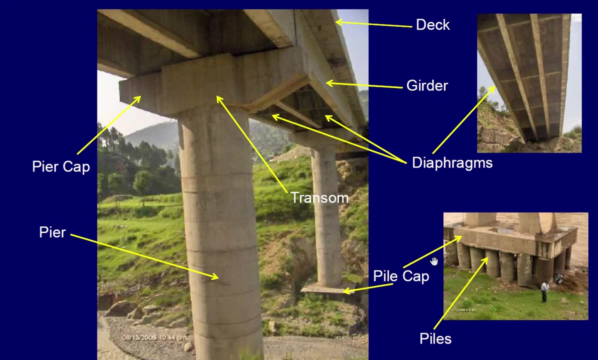 between substructure and superstructure components. now continuing those components. so you can see that these are the piles: the lowest part of the bridge piles, right right here. you can see the piles on the piles. above the piles there is a pile cap. the pile cap is supporting the pier. the pier is then converted into. 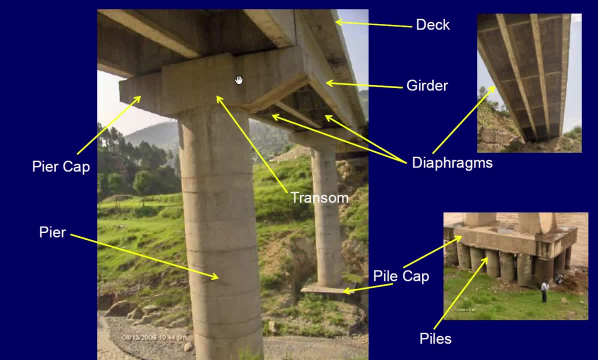 pier cap, the cap of p step, okay, and the pier cap is supporting the girders. these are the girders. the girders are supporting the deck slab. okay, so this is the mechanism. you can see the transom as well. you can see the diaphragms as well. 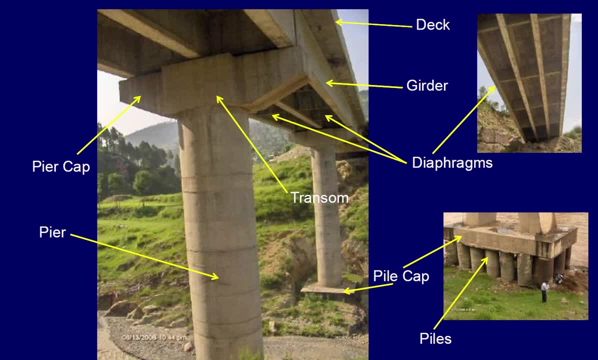 so these are the different components of a bridge, of a typical girdle bridge, not the slab bridge, not the able stirred bridge, not travel bridge. and Wiebalstduino protects the cinnamon proven means, not the cable street 자, not the cable from the bridge, not the table tree from the bridge bridge or the. 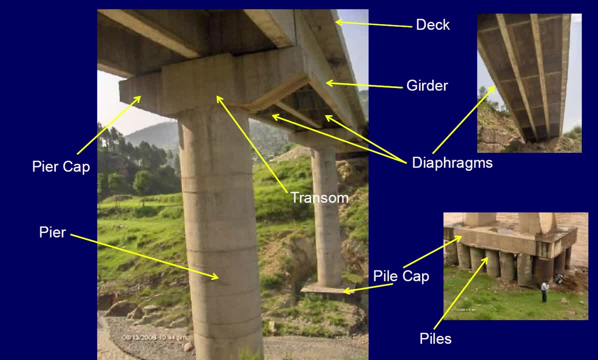 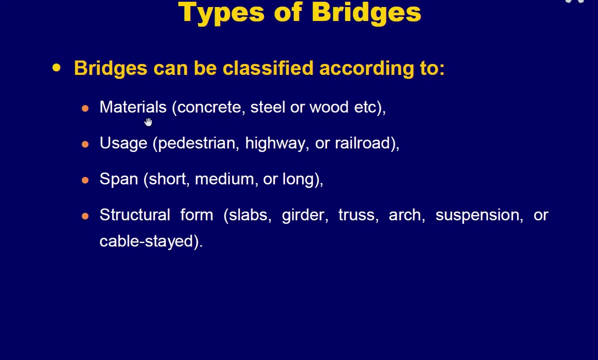 the suspension bridge or other types of bridges, is a simple girdle bridge. so, coming to the point, how many types of bridges are there? bridges can be classified according to materials, for example, made of concrete or steel or wood, etc. usage: what kind of usage it has, for example, the pedestrian. 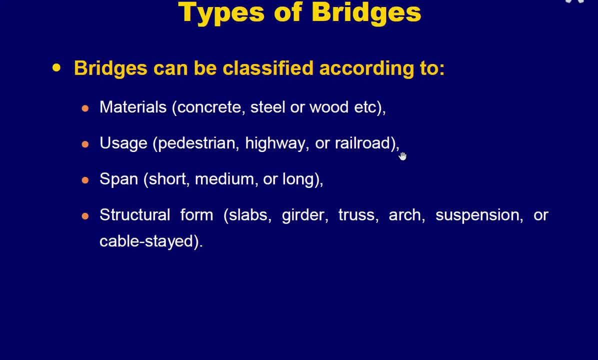 usage or the highway traffic or railroad traffic. what are these spans? for example, short span bridge, the medium span bridge, the long span bridge- usually short span- are girder bridges, medium are cable straight and long span bridges are suspension bridges. structural form: for example slab bridges, girder bridges, truss bridges, arch bridges, suspension or cable straight bridges. okay, 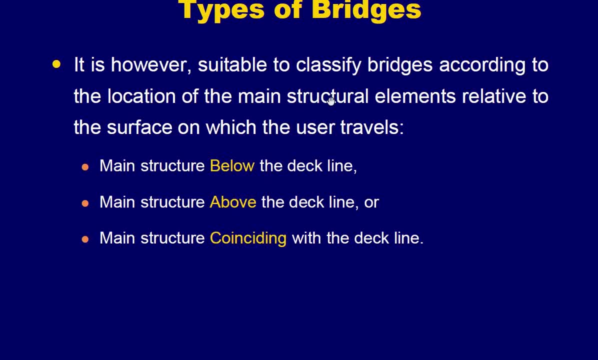 so it is, however, suitable to classify bridges according to the location of the main structural elements relative to the surface on which the user travels. so there is another classification of the bridges according to what the location, for example if the main structure is below the deck line, or if the main structure is above the deck line, or if the main structure. 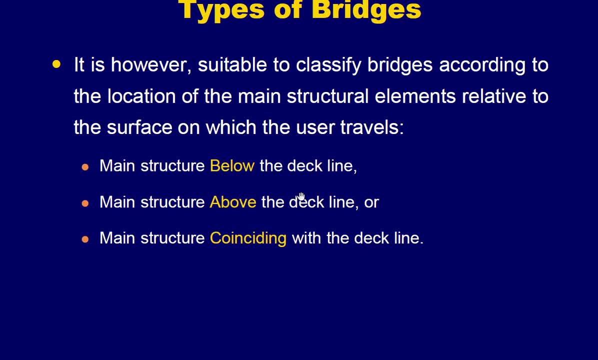 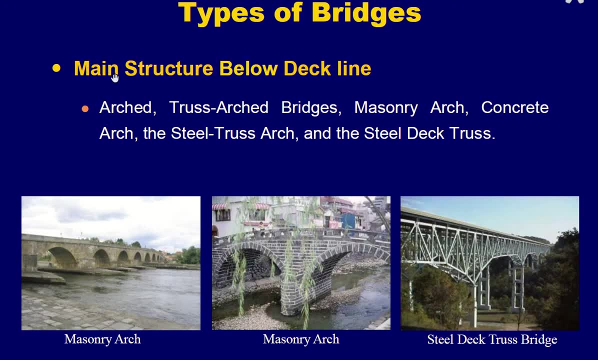 is coinciding with the deck line. so there are three types of bridges on the basis of location of main structural elements, and I will explain in the coming slides. okay, now coming to the first type, when main structure is below the deck line. so you can see the. 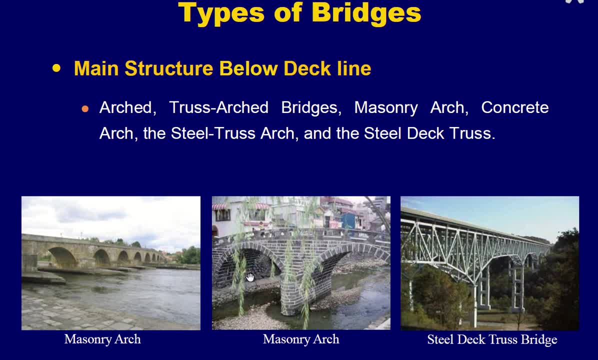 example of arch bridges: see masonry arch bridge, masonry arch bridge and steel deck truss bridge. in all these type of bridges you can see the deck line where the where the people or the cars or traffic travels. so the main structure is below the deck line. deck line is over here and all the 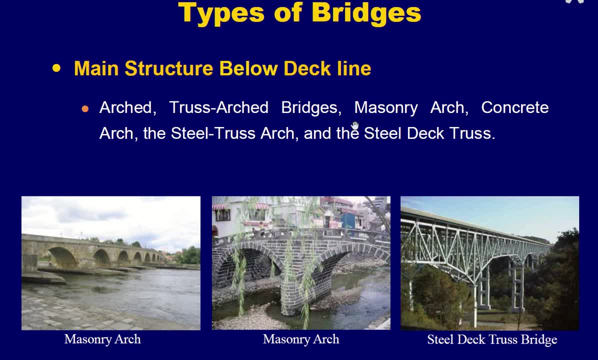 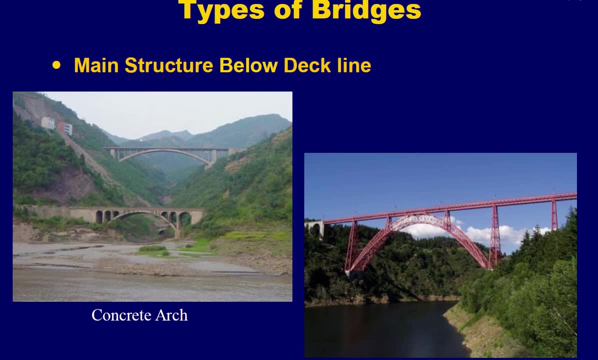 main structure is below this line. so all truss arch bridges, masonry arch bridges, concrete arch, steel arch and the steel deck truss bridges are above the main structure where the main structure lies below the deck line. the second one is when main structural. okay, I'm sorry this is the continuation of the previous slide where different. 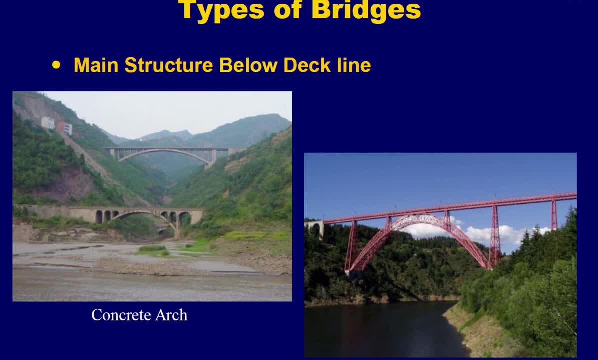 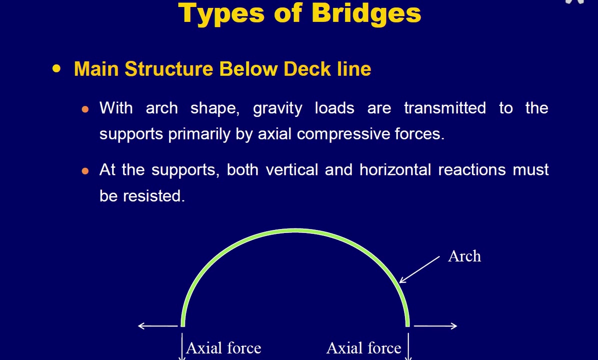 types of bridges are shown where main structure is lying below the deck line. so you can see, or here as well, that all these bridges, the deck line lies above the main structure. right mechanics of main structure below deck line with arch shape, gravity loads are transmitted to the 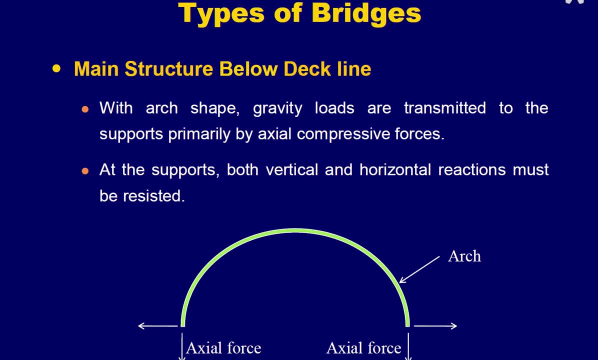 supports, primarily by axial compressive force. at the supports, both vertical and horizontal reactions must be resisted. so this is what you have learned in structural analysis, right, the analysis of arches. so there is a horizontal thrust and there is an axial force, so arch must be designed for that, uh, and both horizontal and vertical reactions must be resisted at the 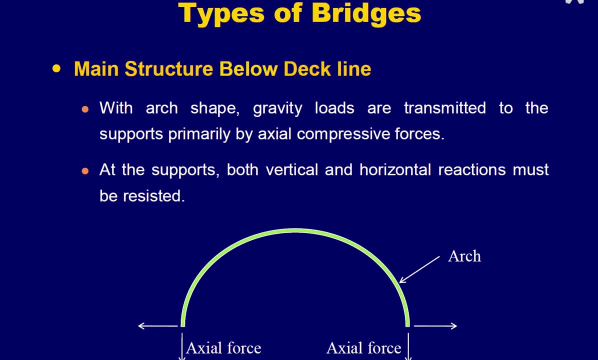 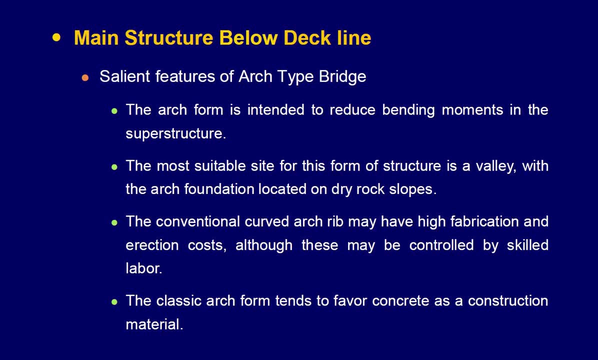 support, so in this case the support must be stiff and strong enough horizontally as well as vertically. some key features of this type of bridge are that the arch form is intended to reduce bending moments in the superstructure. the most suitable side for this form of structure is a valley. the arch form is intended to reduce bending moments in the superstructure. the most suitable side for this form of structure is a valley. the arch form is intended to reduce bending moments in the superstructure. the most suitable side for this form of structure is a valley. 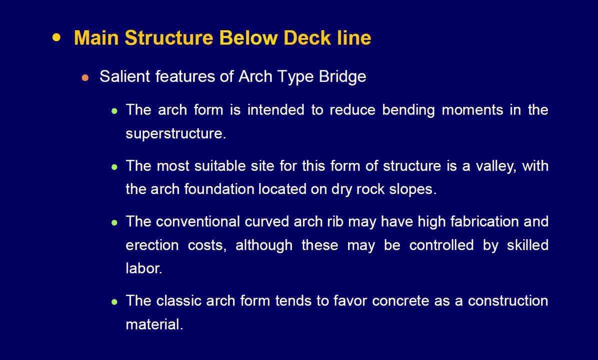 with the arch foundation located on dry rock slopes, because the foundation must resist the horizontal and vertical reactions, so a rock- dry rock- will be a suitable position. the conventional curved arch rib may have high fabrication and erection costs, although these may be controlled by skilled labors. the classic arch form tends to favor concrete as a 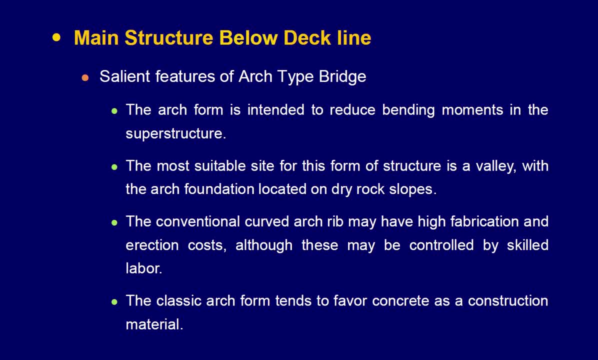 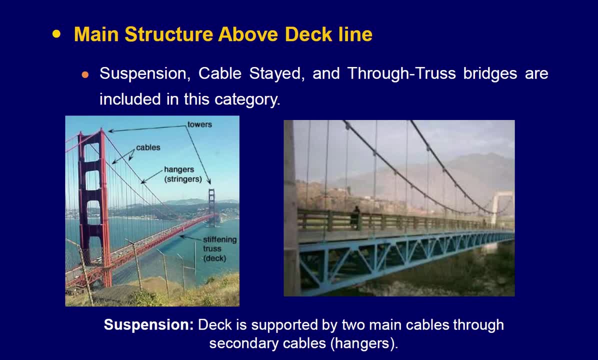 construction material. so these are some salient features of this type of bridge. the other type is when main structure lies above the deck line. so the suspension cable state and through truss bridges are the main examples. you can see the uh, the deck line and you can see the. 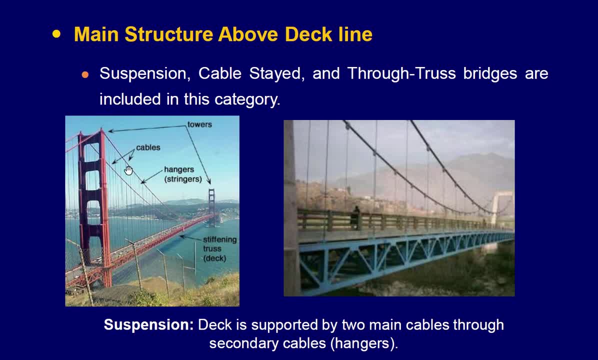 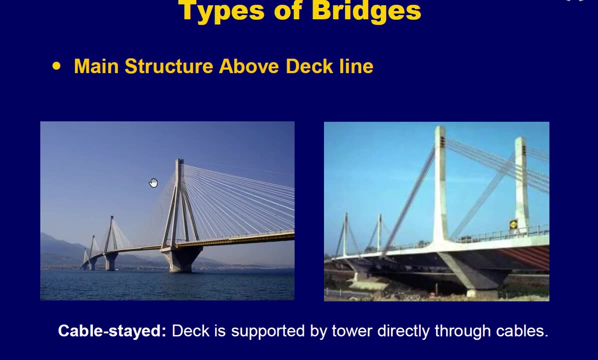 main structure. okay, the main cables, the hangers and the towers. all the main structure is lying above the deck line. this is also a suspension bridge. similarly, cable straight bridges. let me show you that. yeah, see the cable straight bridges. this is the deck line and these are the 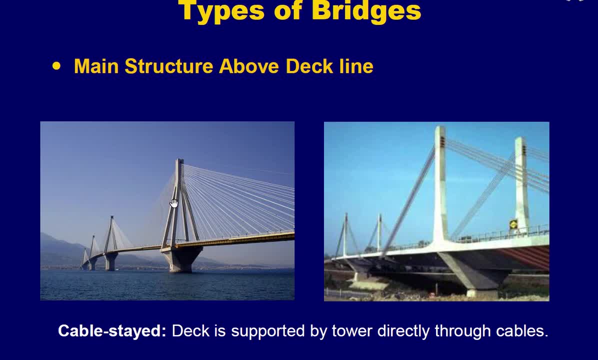 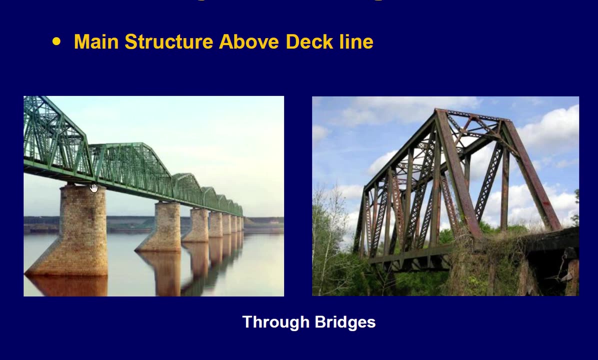 cables and these are the towers. so main structure lies above the deck line, right over here as well, and and the through truss, uh bridges, where you can see this is the main deck line and the trusses, all the trusses, lies above the deck line. so these are the examples of main structure above the deck line right. 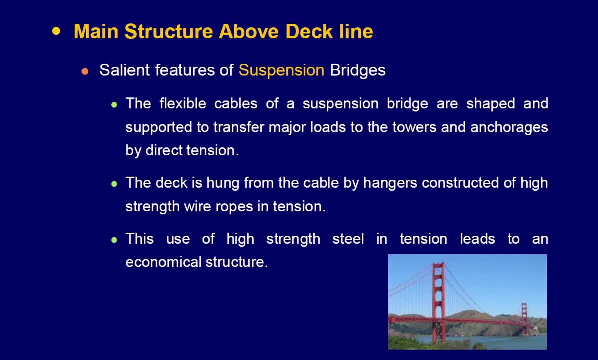 the important features of this kind of or type of bridge is: the flexible cables of a suspension bridge are shaped and supported to transfer major loads to the towers and increases by direct tension. so in suspension bridges, the the deck load is transferred to the cable via hangers and the 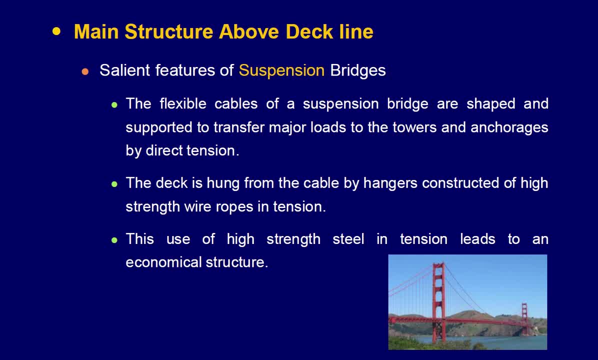 load from the cable to the suspension is transferred to the cable via hangers and the load from the cable is transferred to the anchorages and the towers by direct tension in the cable. the deck is hung from the cable by hangers constructed of high strength wire ropes. intention, as i explained. 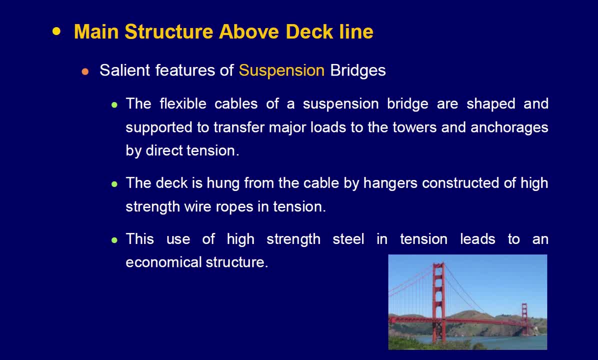 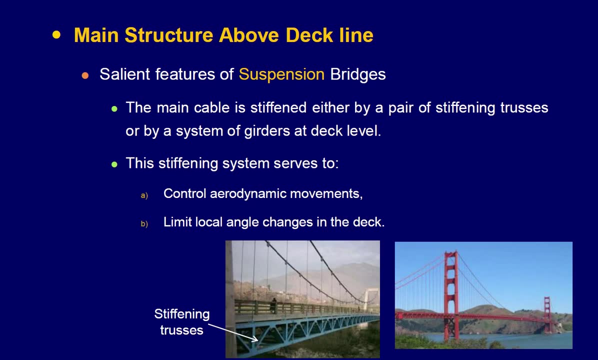 this use of high strength steel intention leads to an economical structure and these are used for the long span structures right, for example, the akashi bridge in japan. it is a suspension bridge. some more features: the main cable is stiffened either by a pair of stiffening trusses or by a 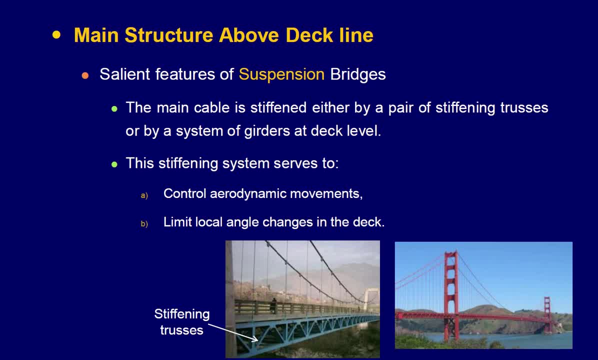 system of girders at deck level right. this is all we are talking about: suspension bridges, one one of a type of main structure above deck line. this stiffening system serves to control aerodynamic movement, the movement of high speed wind and limit local angle changes in the deck. 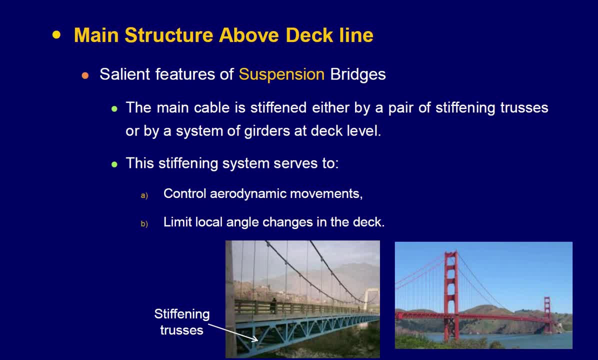 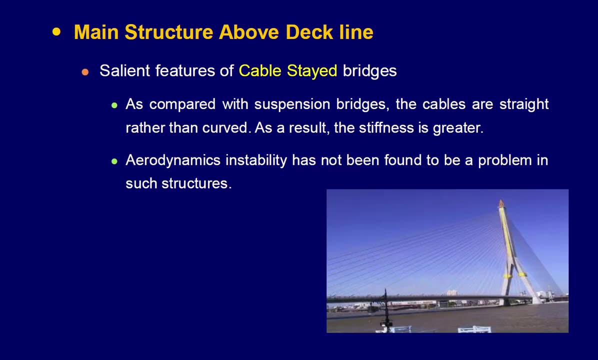 right, the, the stiffness or the serviceability of the deck remain intact during the wind, storms or something like that, or even the passage of the traffic. so you can see how they maintain the, the stiffness of the structure, some important, some important features of the cable state which is, as compared to suspension bridges. these are the. 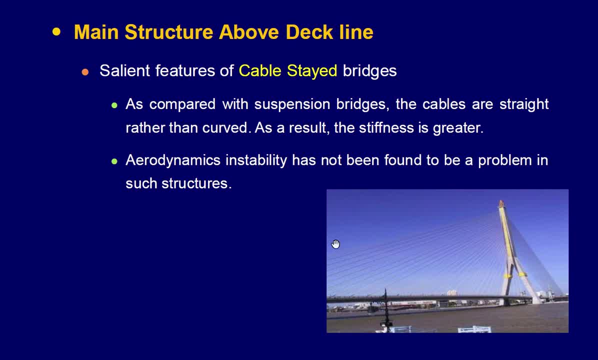 cables are straight rather than curved. okay, in suspension bridges the cable, the main cable, is curved. however, here the cables are straight as a result of the wind, storm or something like that. as a result, the stiffness is greater. aerodynamics instability has not been found to be a problem in 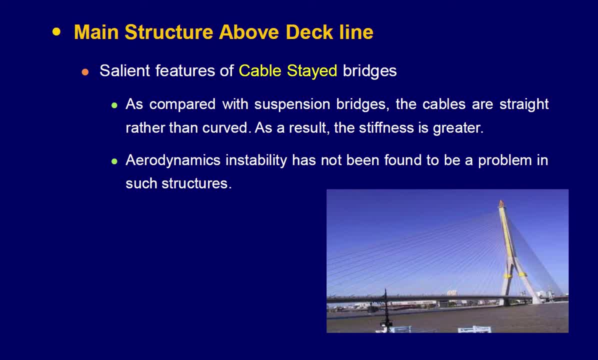 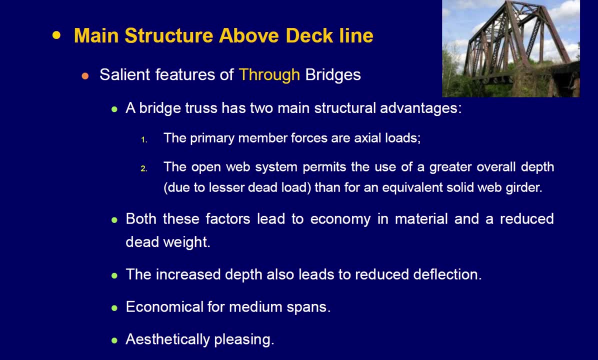 this kind of structure, as we discussed in the suspension bridges- okay- and the through bridges, a bridge truss has two main structural advantages. number one, the primary member forces are axle loads. and number two, the open web system permits the use of a greater overall depth due to lesser dead. 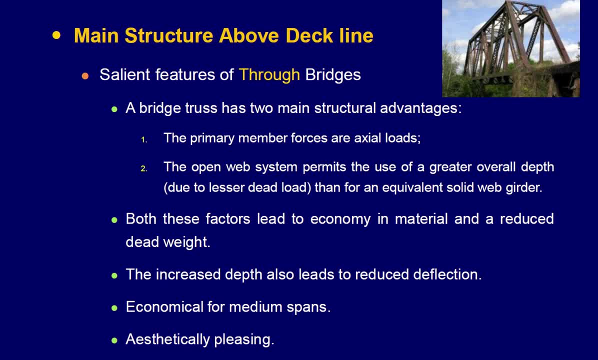 load than for an equivalent solid web corridor. and number three, the two main structure is to allow for long-term construction in a winding loop and the actors lead to economy in material and a reduced dead weight. the increased depth also leads to reduction deflection, economical for medium spans. keep in mind that is not for a 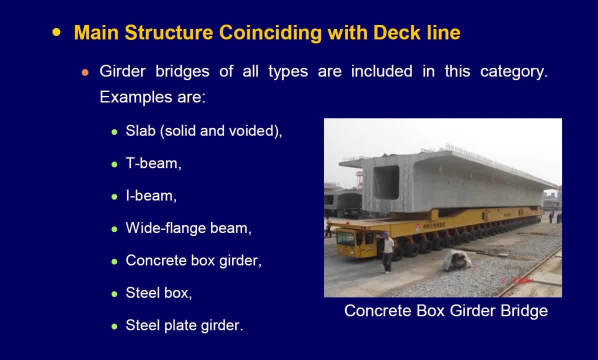 long span structures okay and aesthetically pleasing. these are the some important features of through bridges. the third one is the when main structure conceding with the deck line Goulder. second one was suspension and through bridges and cable street. and third one is the all the. 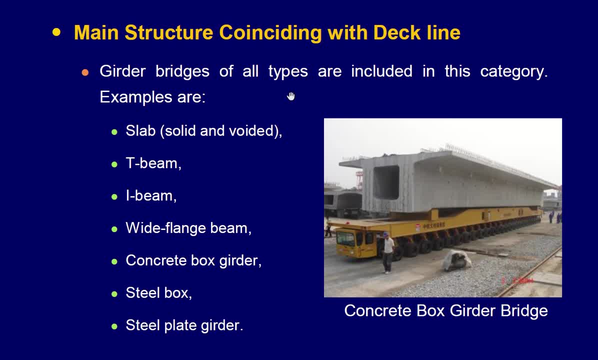 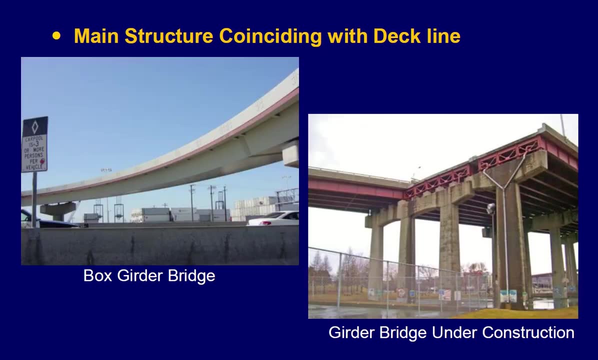 girder bridges right, where examples are slab t beam i beam, wide flange beam, concrete box girder, steel box, steel plate girder- all lies in this category of main structure, coinciding with the deck line right. so you can see very clearly that the main structure, which are girders and the deck, 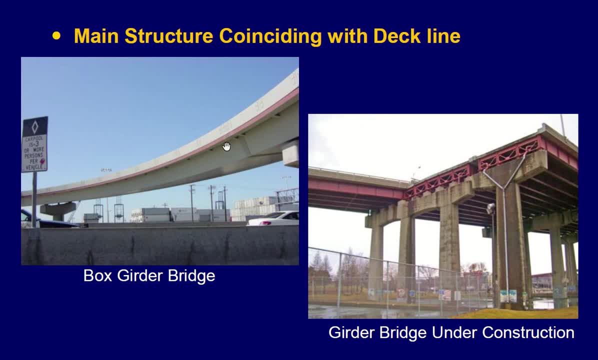 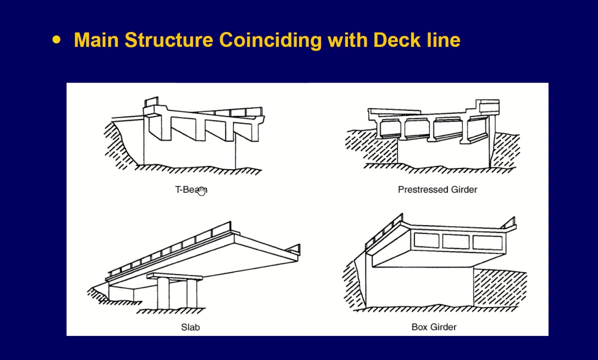 slab in this case lies at the same level: box girder, bridge girder, bridge under construction, where you can see that the eye girder or steel girders are used by the manufacturer and the deck slab. they lies at the same level. so these are different examples, for example, the t beam bridges, the pre-stressed curder bridges, the 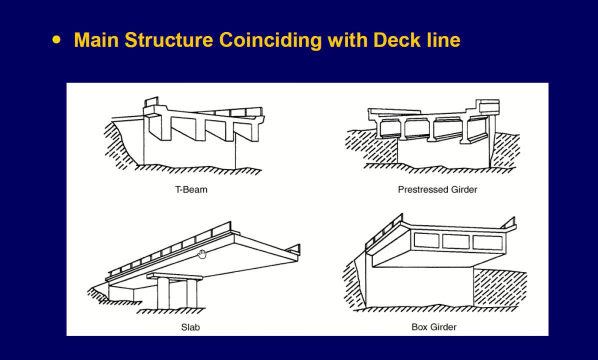 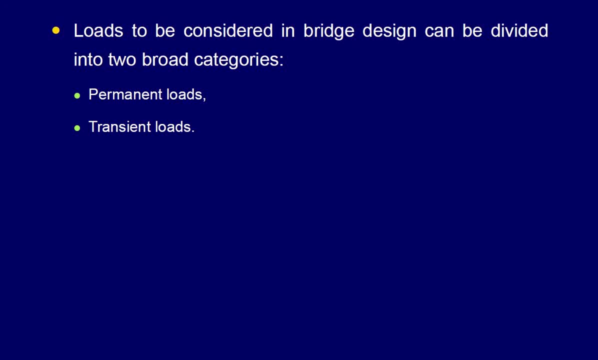 slab bridge- you can see no beam or girder here- and the box curder bridges. okay, now having discussion about the types of bridges, we are coming to the main topic. the loads to be considered in bridge design can be divided into two broad categories: permanent loads and transient. 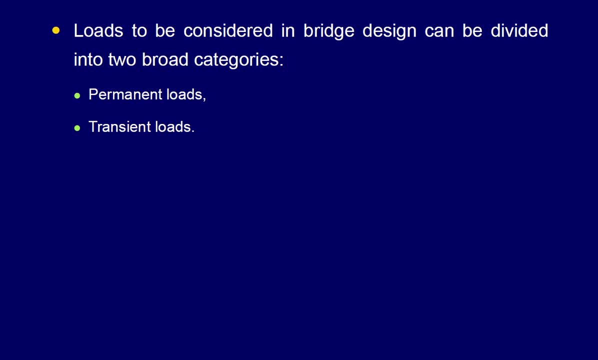 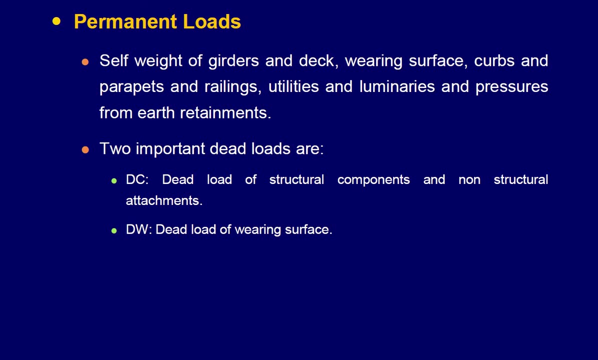 loads, and both are equally important. okay, now taking the first category: permanent loads: self weight of girders and deck wearing, surface curbs and parapets and railings, utilities and luminaries and pressures from earth retainments. these are all permanent loads and will stay there as a dead load throughout the lifespan of the bridge. two: 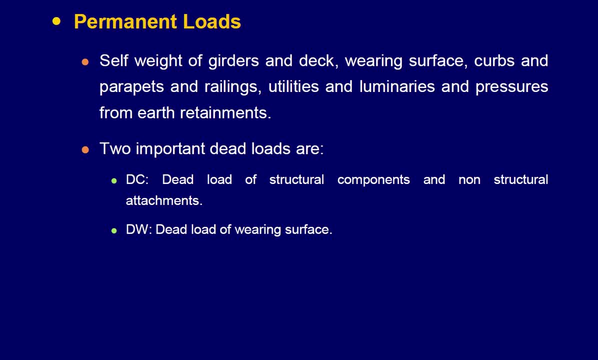 important dead loads are dc, which is called dead load of structural components and non-structural components, and dw, which is dead load of wearing surface. why we are taking it very as different? because the wearing surface may differ at different phases of design life of the structure. okay,